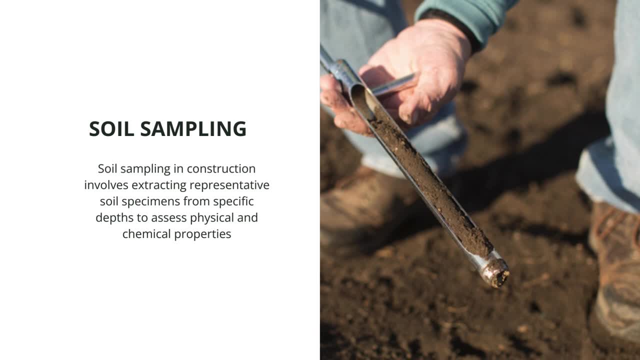 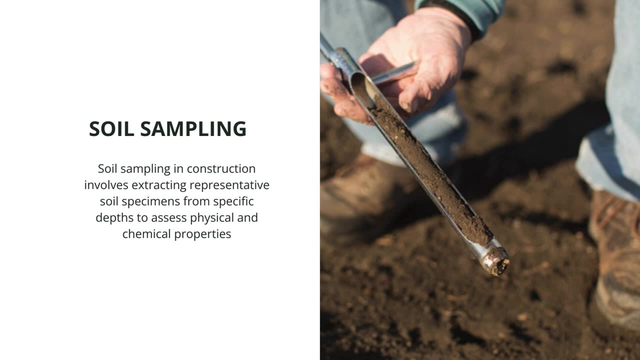 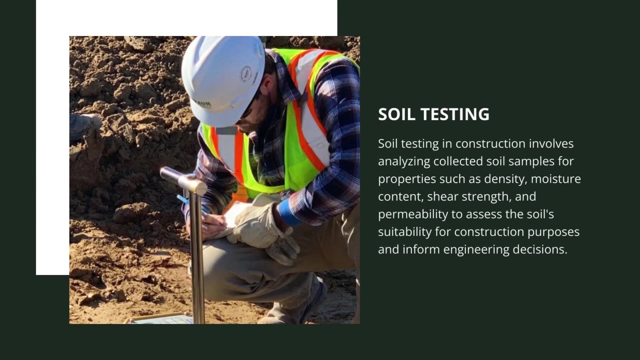 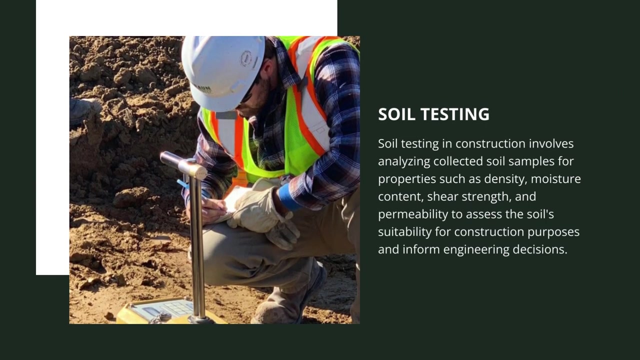 Soil sampling in construction involves extracting representative soil specimens from specific depth to assess the physical and chemical properties, giving an information regarding the foundation design and the construction methodologies. Soil testing in construction involves analyzing collected soil samples for properties such as density, moisture content, shear strength, permeability. 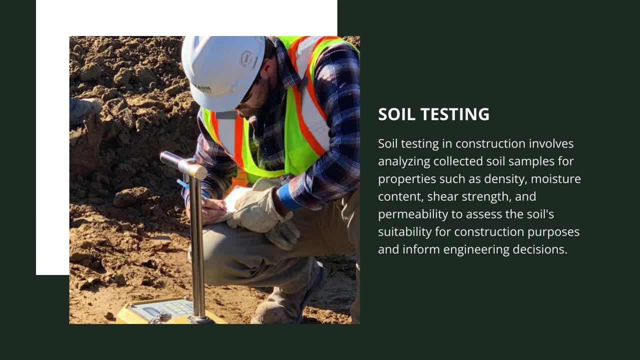 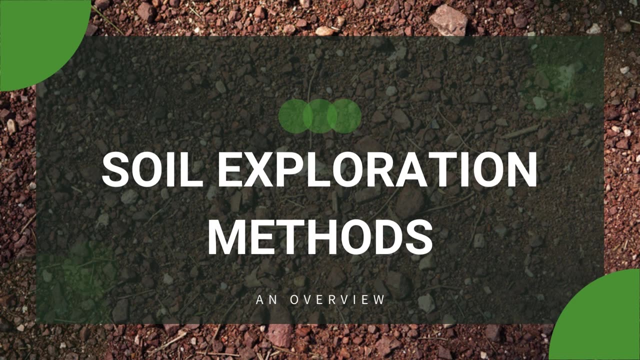 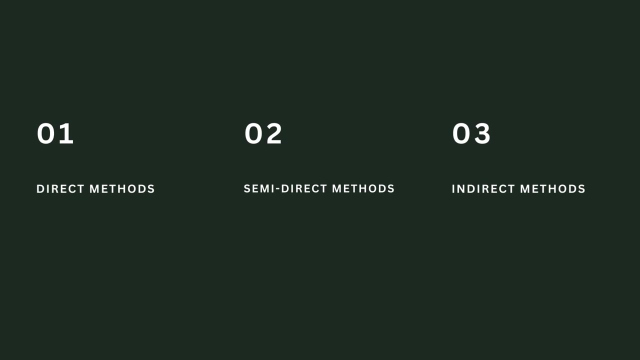 to assess the soil's suitability for construction purpose and inform engineering decisions. So these methods, as I told you, can be either performed together or differently, or simultaneously, and based on which we have different methods of soil exploration. Soil exploration methods can be classified into direct methods, semi-direct methods, 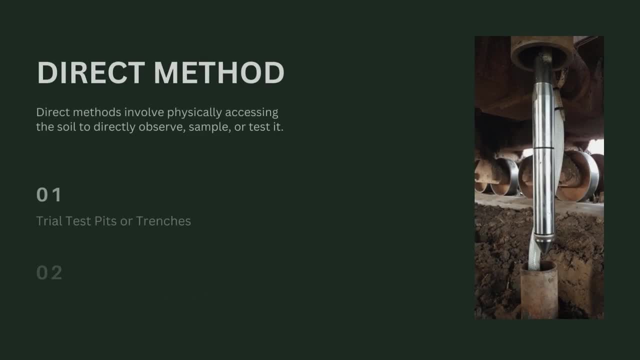 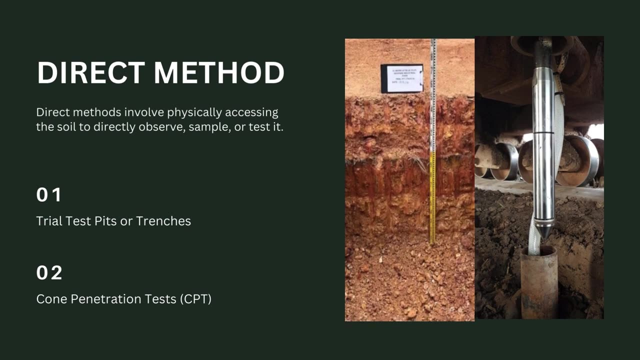 and indirect methods. Direct methods of soil exploration: These are direct methods because it involves physically accessing the soil to directly observe, sample and test it. These include trial test, spit or trenches Cone penetration test Here, as I mentioned, the drilling sampling. 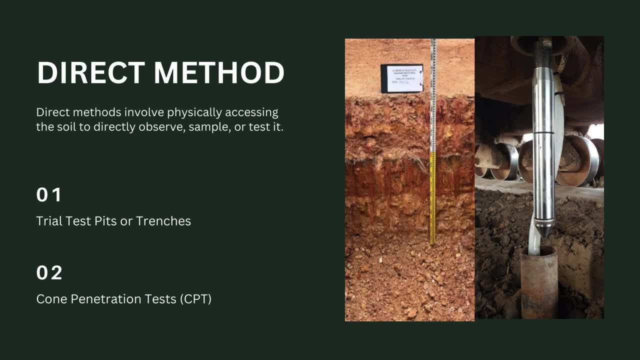 and the testing procedure is conducted simultaneously and the results are obtained directly. 08- Trill Tr救� Stella makes a training operation for 7 days and 2 takes 3 days to perform FCM tests in water. 08- Prima Sem paths are polytrophic and they work atığım north end of the soil in a controlledубor management system, So soil exploration assessment can be done there, or by patient or, as you may, university benefit from Pediatrics. 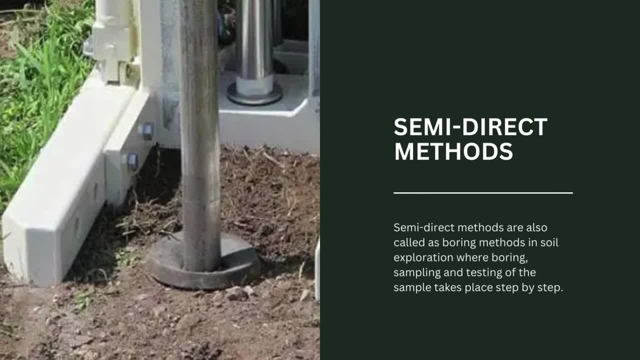 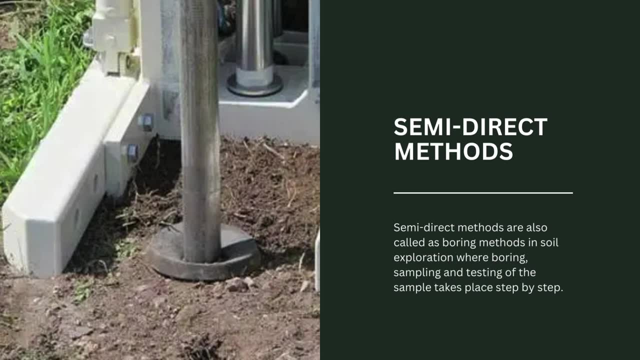 method of soil exploration. Semidirect methods are also called as boring methods in soil exploration, where boring, sampling and testing of the sample takes place step by step. When soil has to be explored at a larger depth, we go for boring methods where use special equipments to bore a hole at a higher. 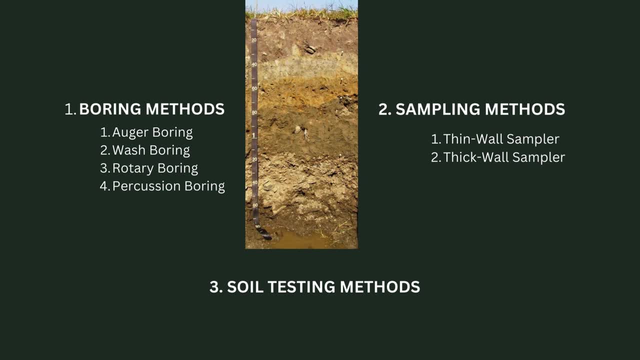 depth to collect the samples. Boring is performed in various methods like auger boring, rotatory drilling, wash boring, percussion drilling, while sampling is performed by different methods and different samplers, like thin-walled tube sampler or thick walled sampler. but you have to keep in mind 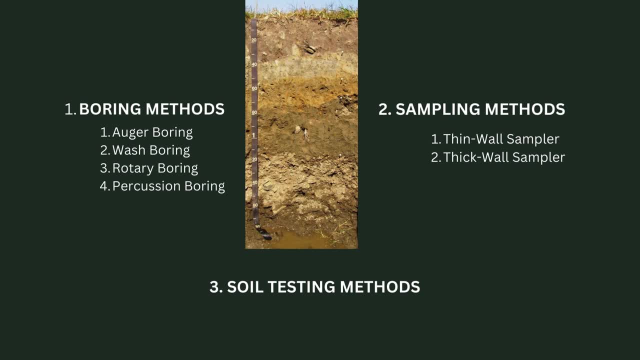 that boring and sampling go hand in hand during the process. What we choose here is the type of sampler that we use with the type of boring machine to collect a sample. After boring and the sampling process we conduct soil testing. As explained before. boring and the sampling methods go hand. 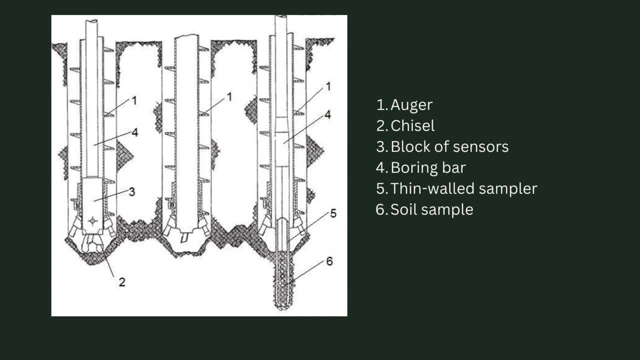 in hand. It can be explained using this figure. This figure arrangement is of all samples- auger boring- where the first arrangement shows how the auger boring equipment is drilling a well inside the strata. after that we remove the sensors and all of the arrangement and the third step is: 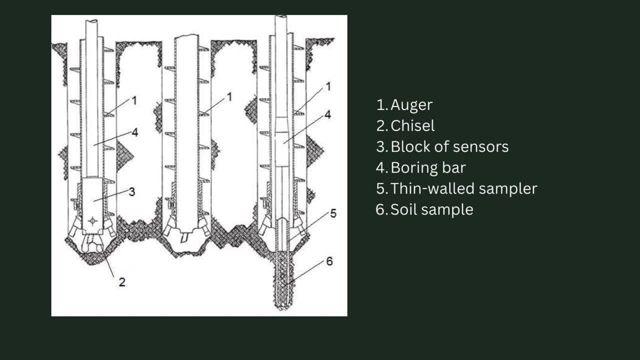 inserting the thin wall sampler- that is, the sampling equipment, that is number five- into the strata where the sample has to be collected. so once the sampler is being inserted down to the strata, the sample- that is number six- is collected into the sampler and we pull back upwards so that 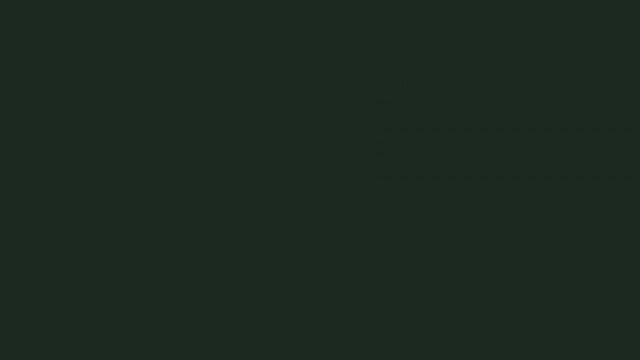 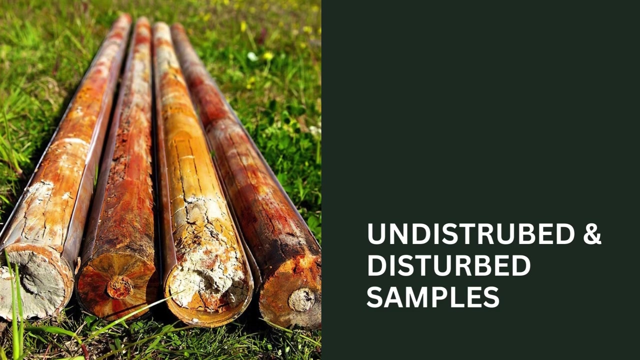 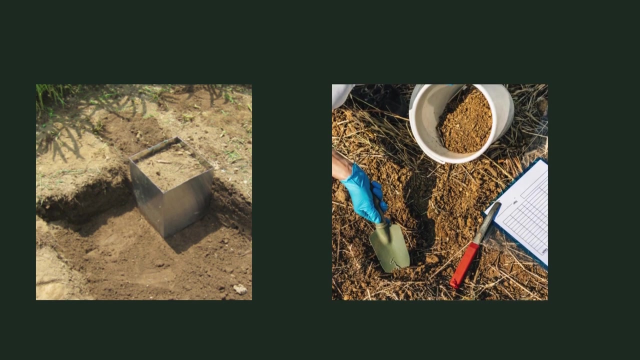 we collect the sample. the samples collected can be disturbed samples or undisturbed samples. now this differs based on the boring method that is selected for procedure. some boring methods give disturbed samples, while some give undisturbed samples. some boring methods collect sample by completely disturbing the soil underneath. 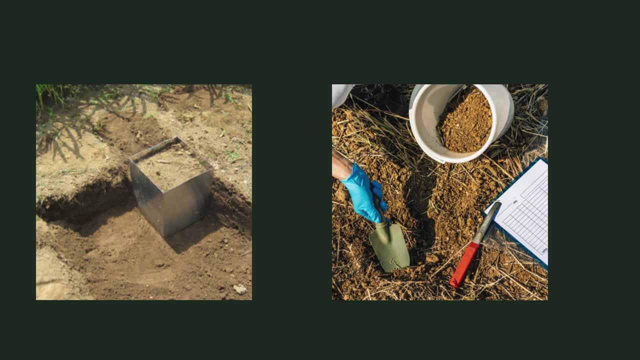 but some drilling machines. they collect sample without disturbing the soil straighter undisturbed. the type of boring method, sampling method, sample type and the test conducted are also dependent on the type of the soil straighter, as we are talking about semi direct method. once we have 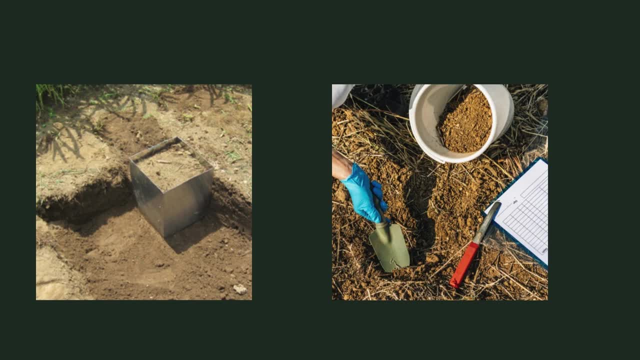 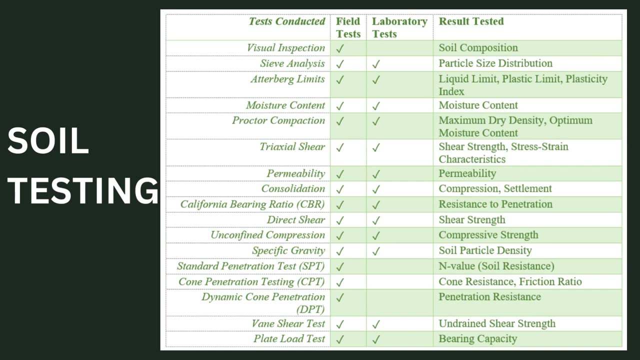 collected the samples, we undergo that sample for soil testing. there are numerous tests that can be conducted on soil once a soil sample is collected. some of them has been categorized on the table as shown, starting from visual inspection. that is the one test- direct test- that I've explained before. we have 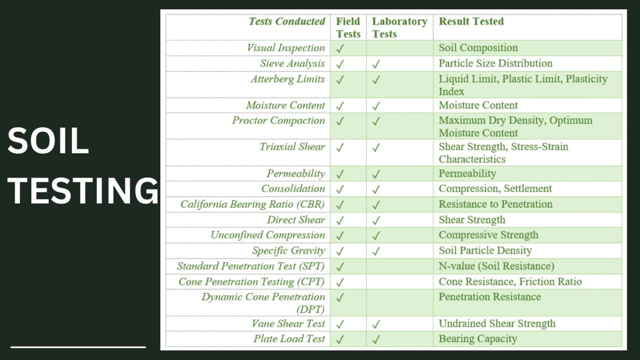 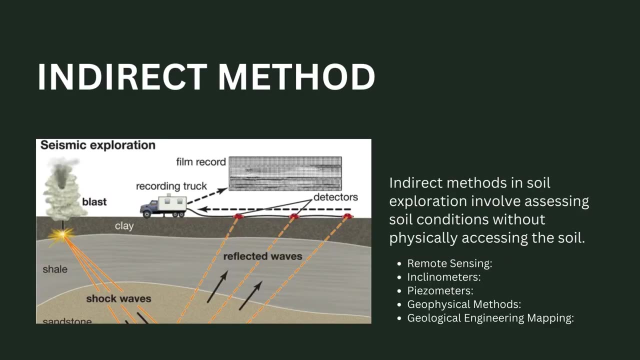 sieve analysis at a book test, moisture content test, proctor compaction test and we have standard penetration test, dynamic corn penetration test and Wayne shear test. these are the list of tests that can be conducted on the soil during soil exploration but one are the entire egg methods of soil exploration, entire. 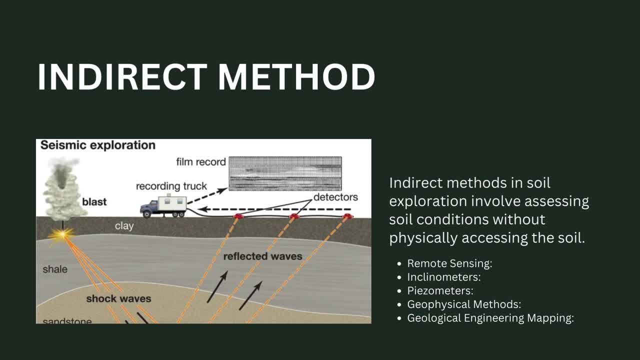 egg method in soil exploration involves assessing soil conditions without physically accessing the soil. these methods relevant to soil exploration and soil exploration and soil exploration and soil on measurements, observations or data collected from the surface or the surroundings to infer information about the subsurface. some common methods include geophysical methods, remote sensing inclinometers, piezo meters and. 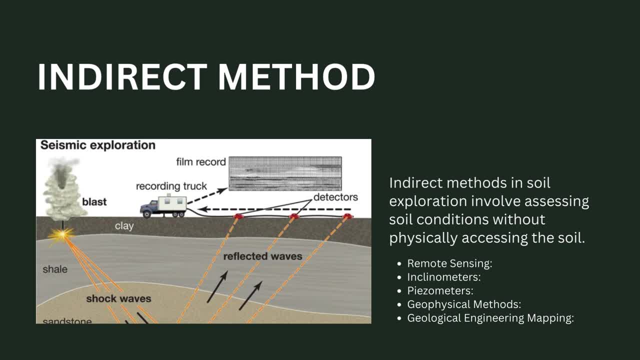 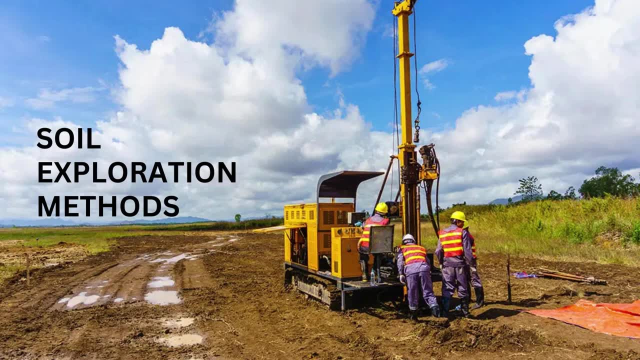 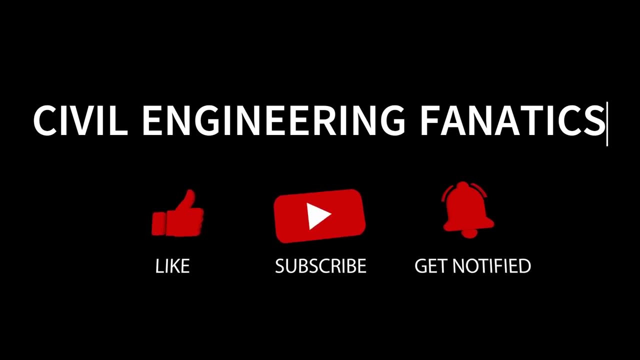 geological engineering mapping. we believe you have gained a comprehensive understanding of the diverse category of soil exploration methods. stay tuned for the detailed videos on each of these methods. make sure to subscribe to our channel for more information. civil engineering and construction videos.